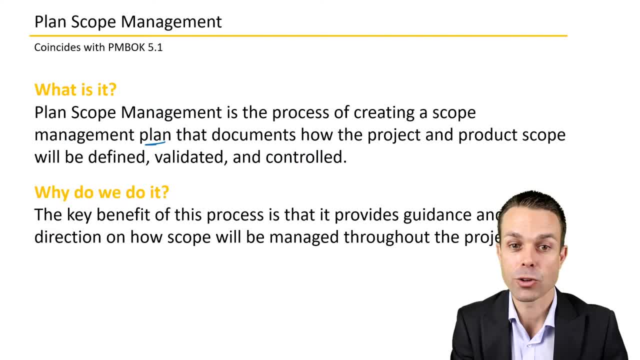 is the process of creating a scope management plan, The documents, how the project and product scope will be defined, validated and controlled. Those three things very important. How are we going to define the scope, How are we validating that it's correct And how are we going to? 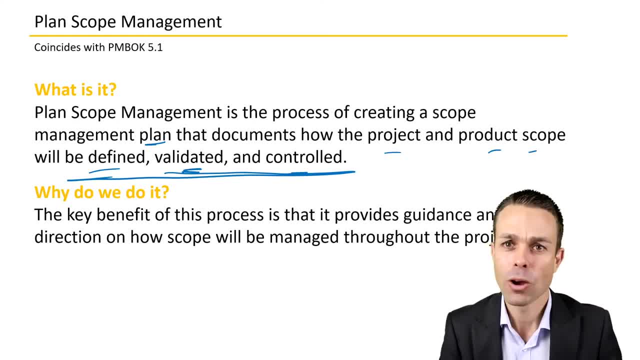 be controlling it to make sure that it stays on track. Why do we do this process? Well, it provides guidance and direction on how the scope will be managed throughout the project, And this is very important. I've seen it many, many times where a project will not have a process. 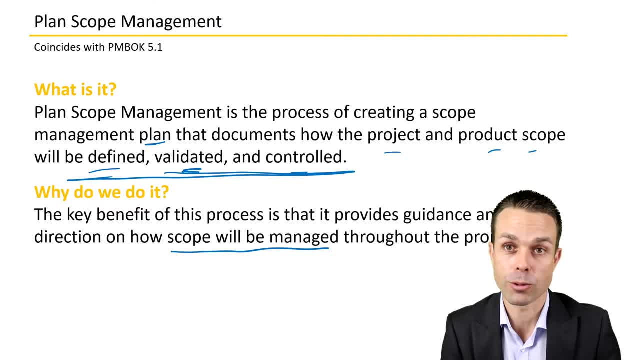 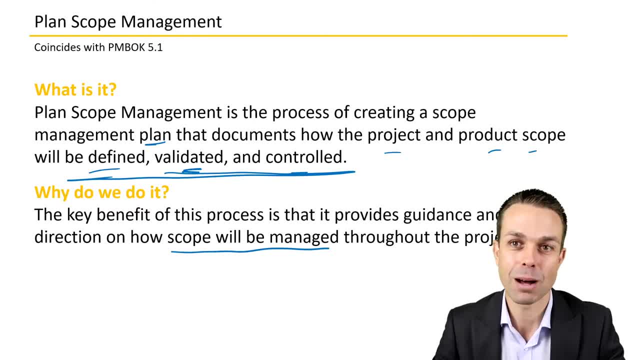 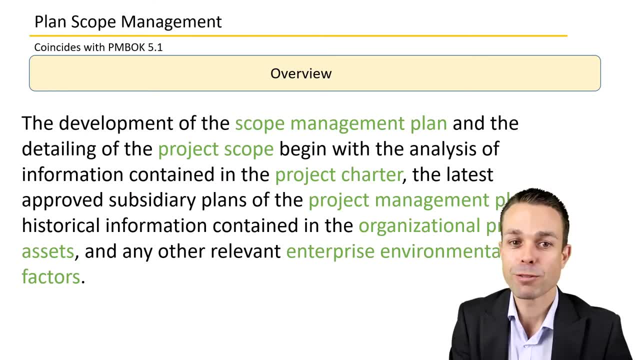 very, very, very, very, very, very feasibly go off track. So if you have a plan up front, it's going to help you a lot more, and if it's outlined and everyone is clear, that's going to help you a lot more again. So the development of the scope management plan and 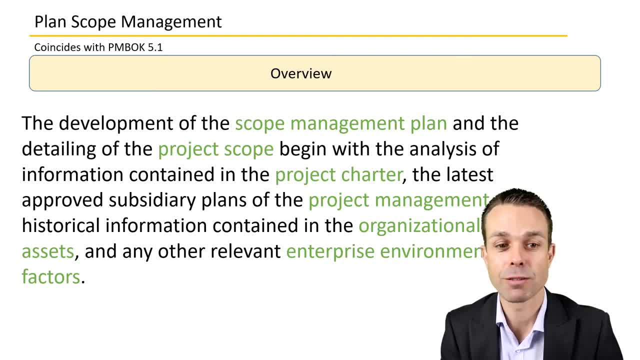 detailing the project scope begin with the analysis of information contained in the project charter. So that's our initial document that we use to initiate a project or kick off a project, and it will have an idea of what we wanted to deliver in the first place. but 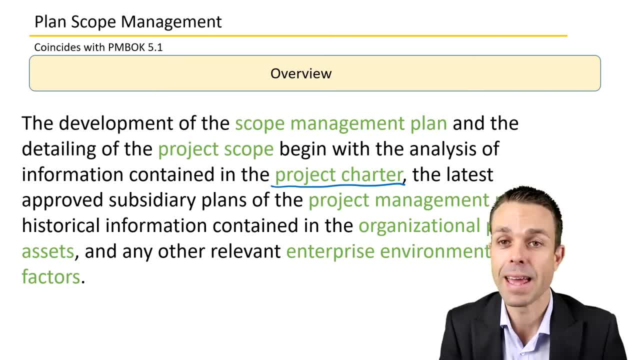 it won't be really well defined. defined, it'll be a high-level idea. now is the time that we're going to start getting into more detail: the latest approved subsidiary plans of the project management plan, historical information contained in the organizational process, assets and any other relevant and environmental and enterprise. 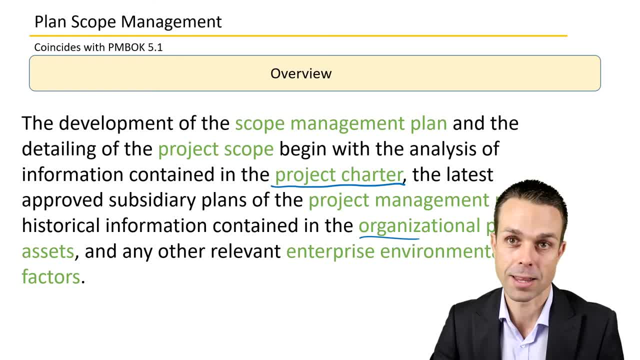 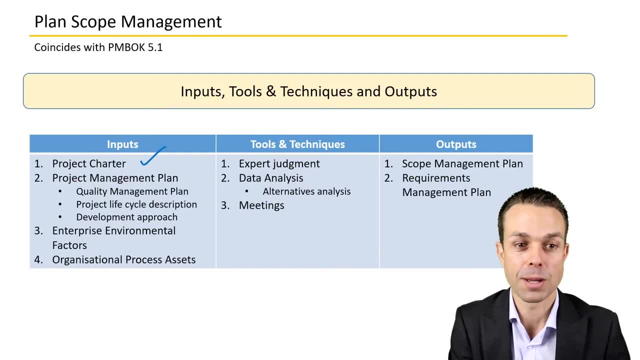 environmental factors like regulations or government regulations or standards and that sort of thing. inputs, tools and techniques and outputs for planning scope management we've got the project charter will need to be an input. the project management plan will be an input into this and it will be ongoing. 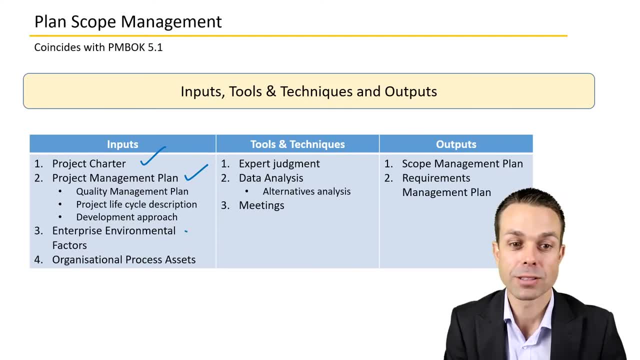 as we're evolving over time, EF's and OPA's, of course, tools and techniques that we'll use, our expert judgment of people in various areas, maybe the customer as well, where we're actually going to be delivering this item, or gathering the requirements from data analysis. so there might be alternatives. 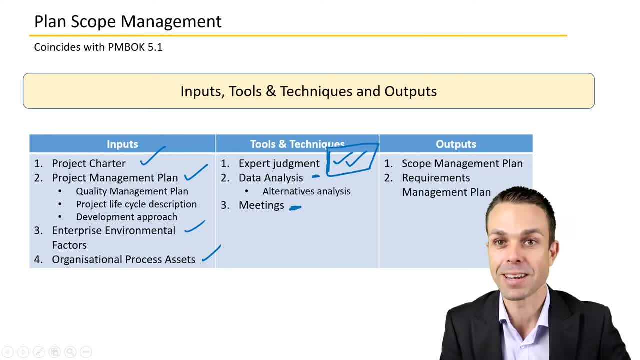 to choose from, and we'll need meetings to facilitate and elicit all of this information from the people that we need you. the outputs are the actual scope management plan, or the requirements management plan as well, which is sometimes called the business analysis plan, and basically, with the rise of the business analyst role, you might be. 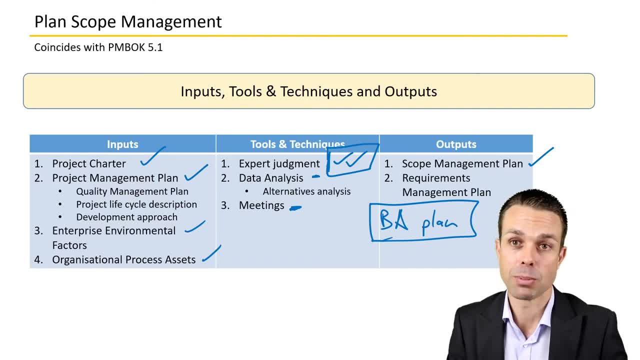 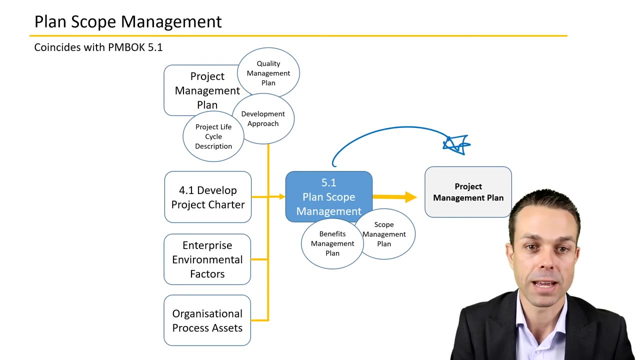 working with a business analyst and they might be doing this particular plan and that will outline how they're gathering those requirements and how they're managing those requirements as the project goes along. as you can see, the plan scope management goes is an input into the project management plan and charter project management plan. 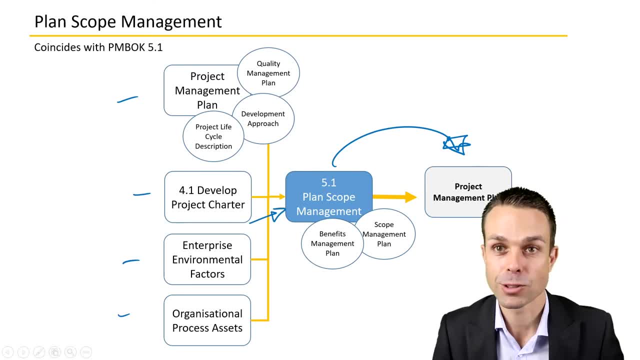 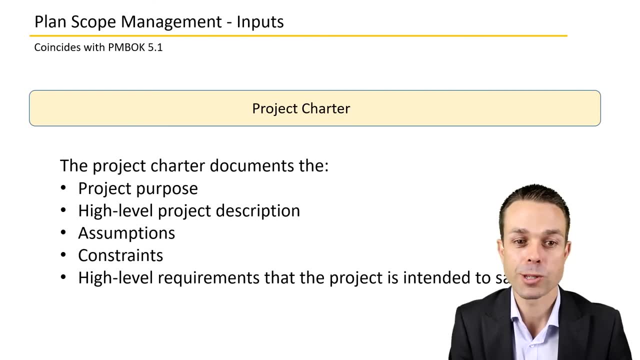 EF's and OPA's are an input into plan scope management. let's look at the inputs in a little bit more detail. the project charter will see. we want to know the project purpose. so what was the actual high-level purpose? the high-level project description? because this will sort of give us a direction on how and 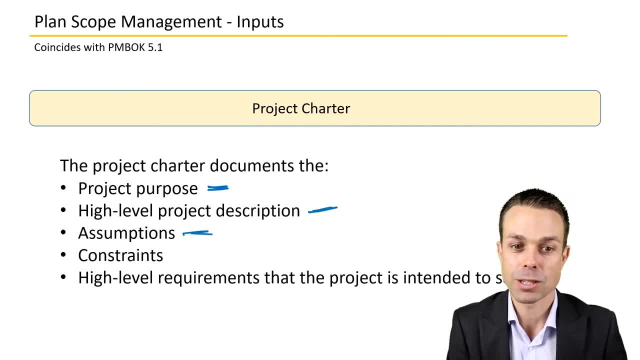 where together those requirements, any assumptions that were made. so you know, maybe we assumed that the project is a project management plan, but we might be that something would be easy to get access to. maybe it's actually hard to get access to. we definitely need to know what we assumed when we initiated this project, any constraints that were. 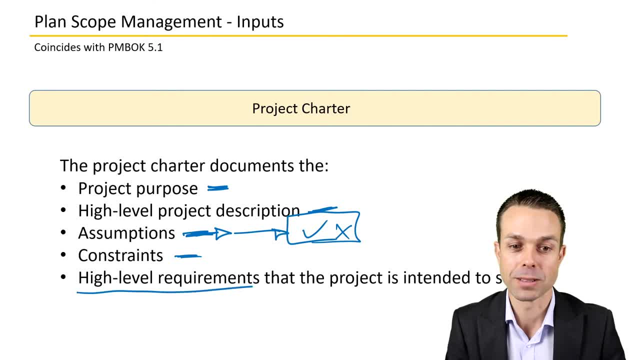 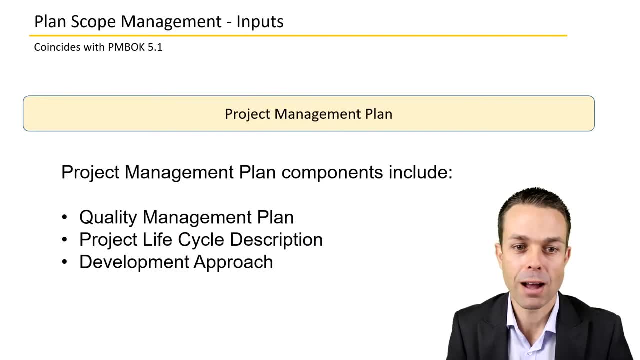 outlined in the project charter and high level requirements that were outlined when the project kicked off with the project charter. the project management plan itself will be an input into this and we'll have the quality management plan. so, with our scope and where, when we're testing our scope, 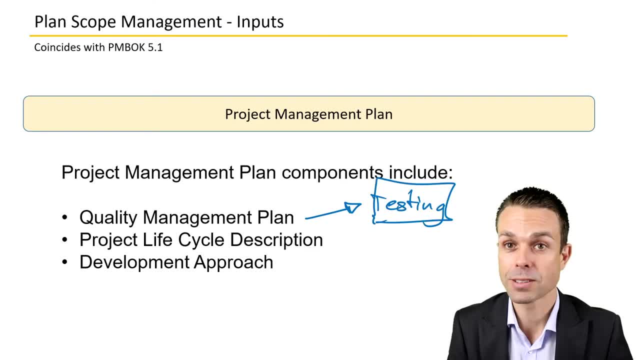 how did it go? uh, was. was it passed? did it meet all of the things that we wanted it to do? were there any defects? this will need to feed back into our planning scope management. we'll also need to know the development approach and project life cycle description. so, are we using agile or are we using? 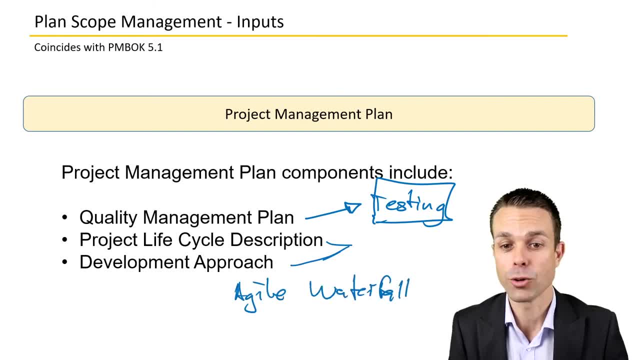 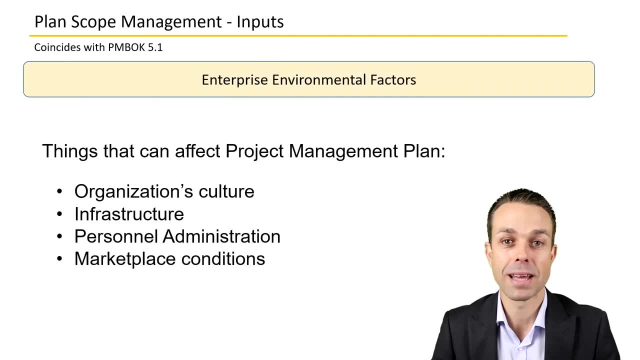 a waterfall approach, are we using a combination of the two, and that will affect how we actually move forward and how we do the work. eefs for project management is a very important tool. planning, scope management include the existing organization's culture. this will affect things. so you know how is the work done? is it done through formal, formal templates or a project? 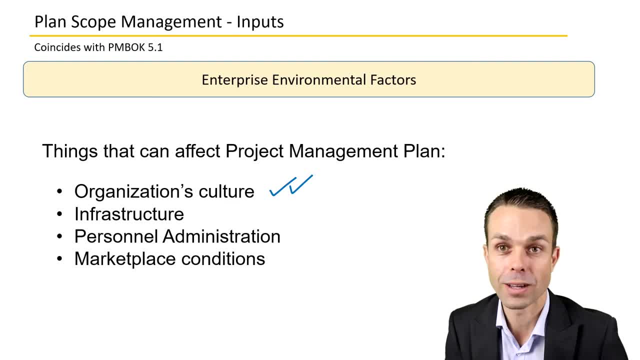 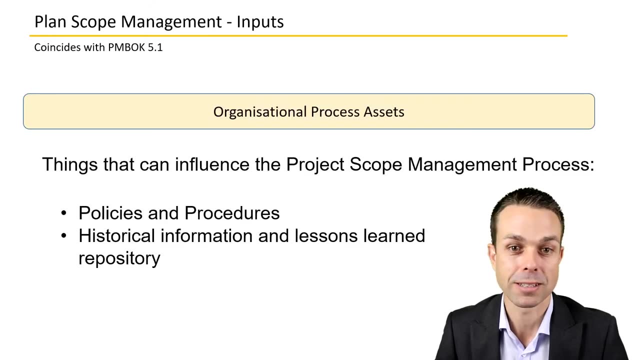 management office or is it done through side or hallway conversations? the existing infrastructure and systems that are in place, any programs that are in use already, personnel administration- how are we getting the resources for our project? and existing marketplace conditions that might affect us. organizational process assets and templates might include policies and procedures often. 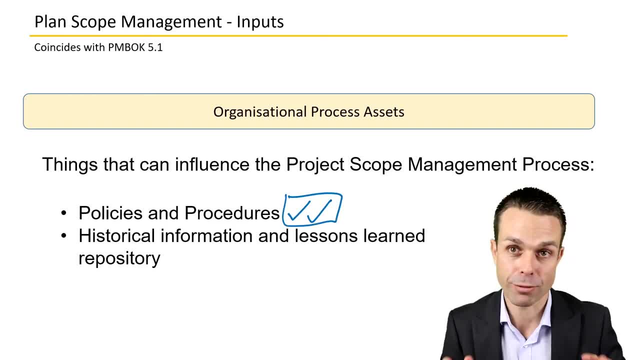 either in a functional management environment where you're delivering the project to, or a project management office that has an idea of the templates that need to be completed, historical information and lessons learned, so previous projects. if you do have a lessons learned repository, then that's a very useful thing. you might get some tips on how something like this was delivered in. 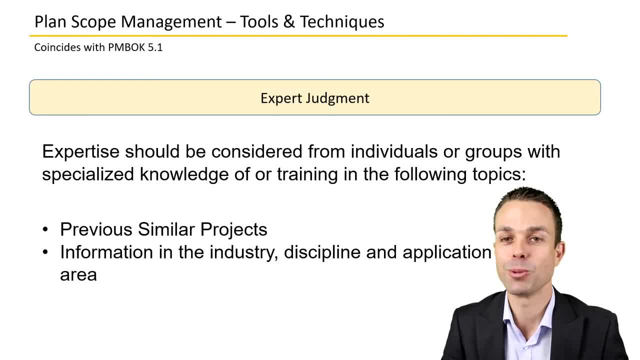 the past tools and techniques for planning scope management. you will need your access to the experts in whatever field you're delving into, so this could be experts on from similar projects. so how, how were things managed on similar projects? can you get an idea from those people and also information in the 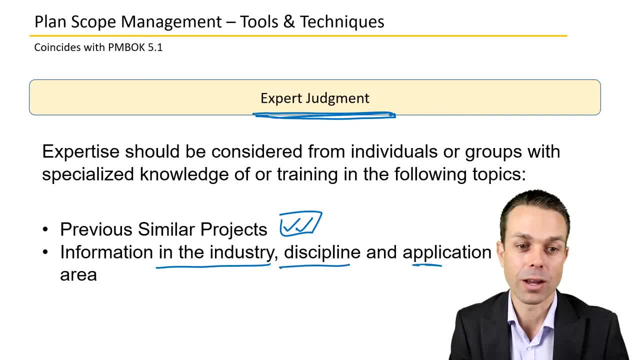 industry or the discipline or the application area, so where you're delivering the product, product to or the project to the people in that area. they're the ex experts in that area and you might need to gather a lot of that expertise through the process of planning scope management. 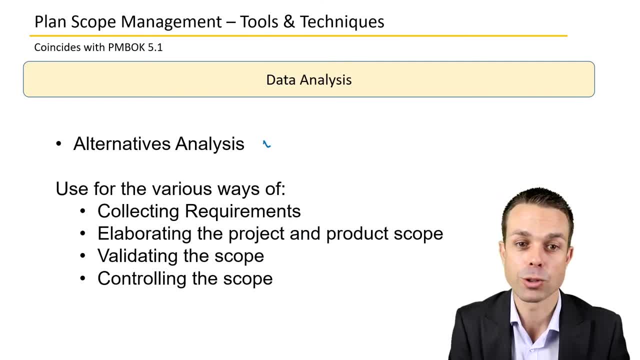 data analysis will come into play, so there'll be alternatives to choose from. you might have a few different solutions as you go along and you'll need to know how to analyze- or how you're going to analyze- those alternatives you can use for the various ways of collecting requirements: validating the scope, controlling the scope or elaborating the 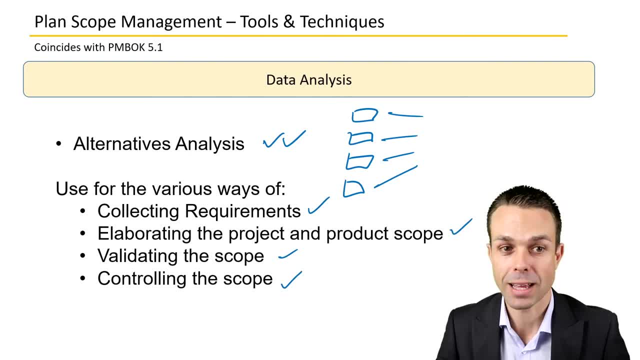 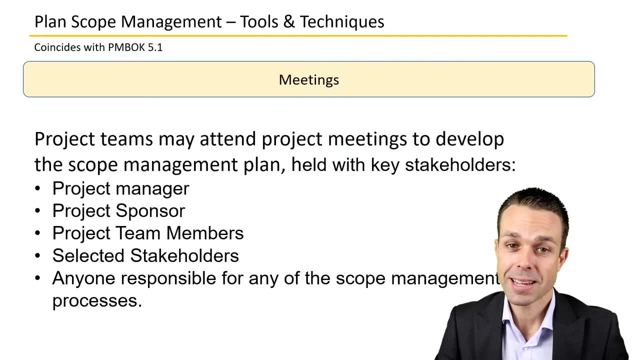 project and product scope, so there'll be- there'll always be- various ways of doing that, and you'll just need to analyze those and choose the best one for your particular particular project. of course, to facilitate this, you will need meetings, one of the easiest and fastest ways when a meeting is run. 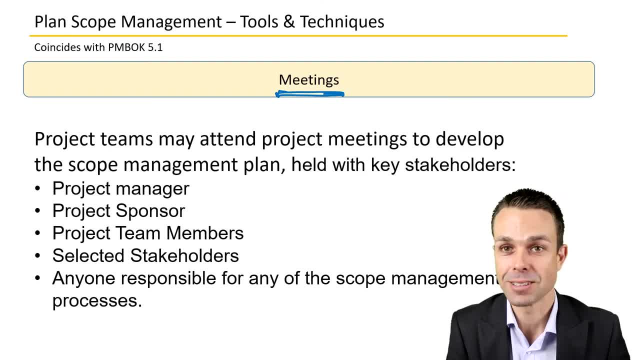 well, you can get an answer very quickly or get decisions and and even gather those requirements very quickly as well. so project teams may attend project meetings to develop the project scope management plan held with key stakeholders, for example, a project manager, project sponsor, project and selected stakeholders or anyone responsible for any of the scope management processes, like 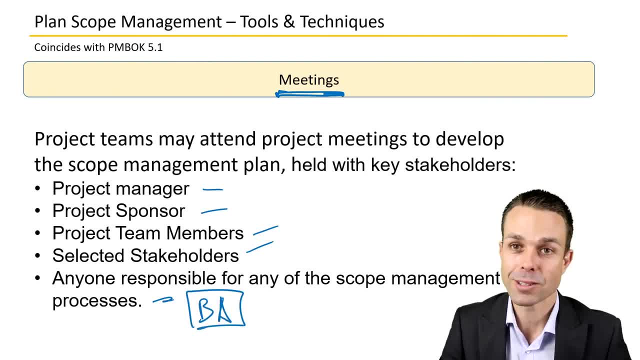 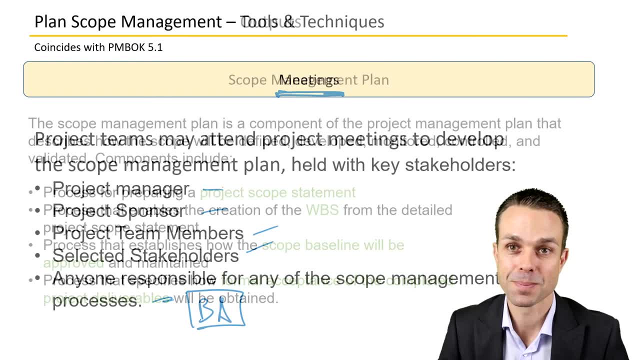 your business analyst role, for example. we'll all get together and agree what is the process for gathering the requirements and making sure that they meet what the customer wants. now there are two outputs you'll see as part of planning: scope management, and we've got the the scope. 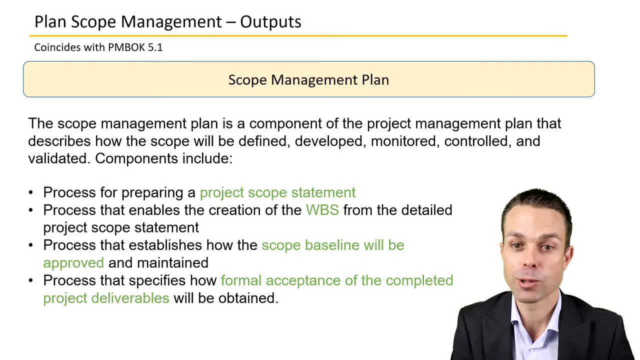 management plan itself. so that's the component of the project management plan. now this becomes a piece of the project management plan right up here, and then you've got other pieces, of course, like risk, cost schedule, quality, procurement and all those things, and it describes how the scope will be defined, developed. 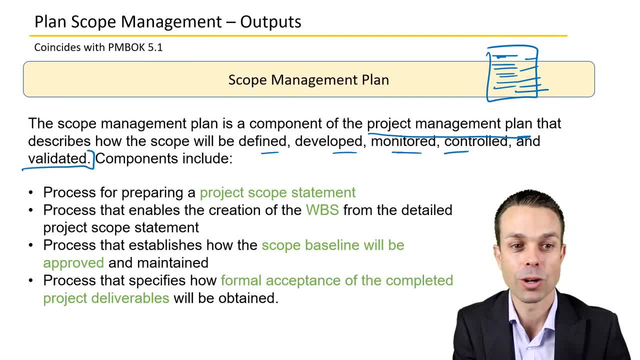 monitored and controlled and, of course, validated, to ensure that the customer got what they wanted. components of this plan include the process for preparing the project scope statement. so we're going to make a statement about what we're delivering and you know what's the process for preparing that, the process that enables the creation of the work breakdown structure from. 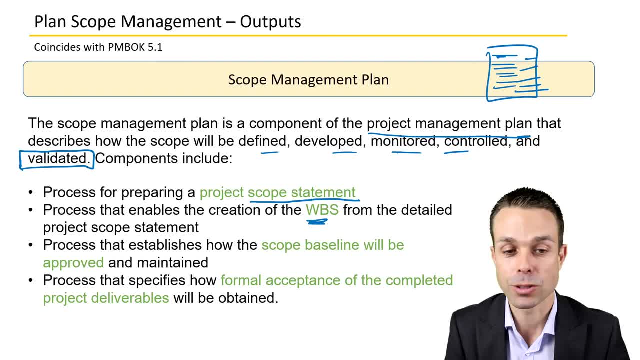 the detailed project scope statement. how are we going to do that? how are we going to break down that scope into the activities? is it going to be a meeting? is it going to be one person doing it? you know who's who's responsible for doing that. all of that can be outlined here. 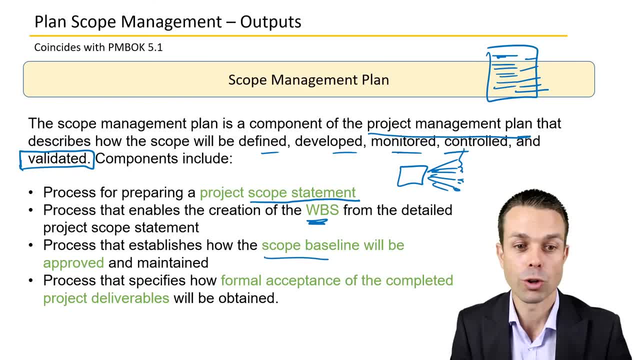 we need the process that establishes how the scope baseline will be approved and maintained. who's going to be approving it? is it the project sponsor? does it need to be run past a steering committee? all of those things can be answered here. pro a process that specifies how formal. 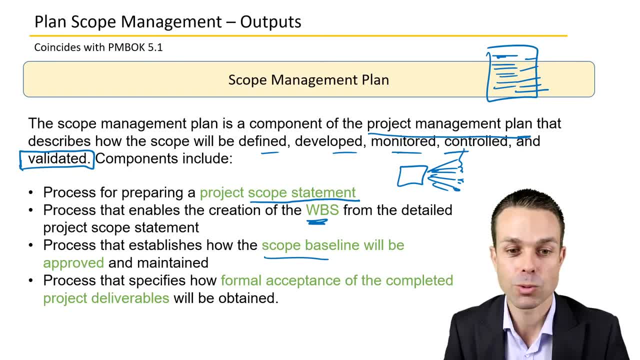 acceptance of the completed project, deliverables will be obtained. so this is where we've got validate scope. that's that process and basically, how do we want that scope to be validated? how do we make sure that it meets what our customers want? lastly, we've got the requirements management plan. 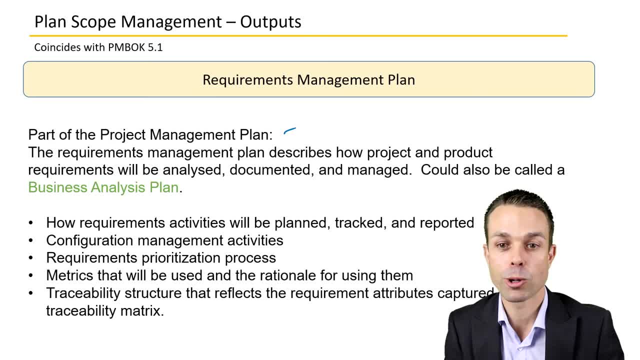 and this is part of the project management plan and it describes how project and product requirements will be analyzed, documented and managed, and it could also be called the business analysis plan because of the rise of that ba role. this is where the ba or the business analyst might come on board and really take this under their wing.